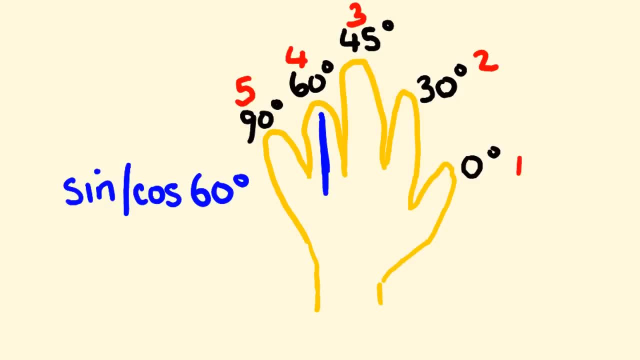 And we're just going to do a couple of things with them, which is as follows: We're going to get the value we see and we're going to square root it and put it over 2.. So I'll show you what I mean. 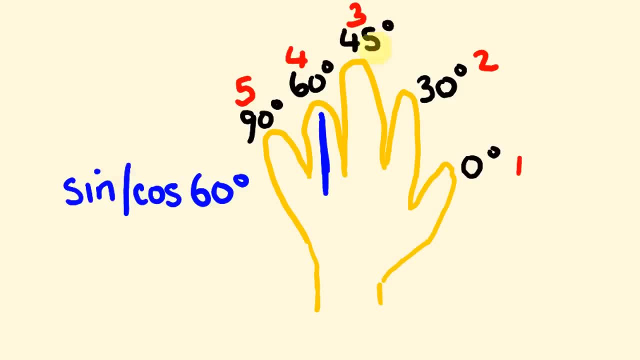 To say cosine of 60, sorry, the sine of 60, it's this: 1,, 2, 3 fingers here. Okay, On that side there's 3 fingers. So I get 3 fingers. I'm going to square root them and I put them over 2.. And that's our answer. 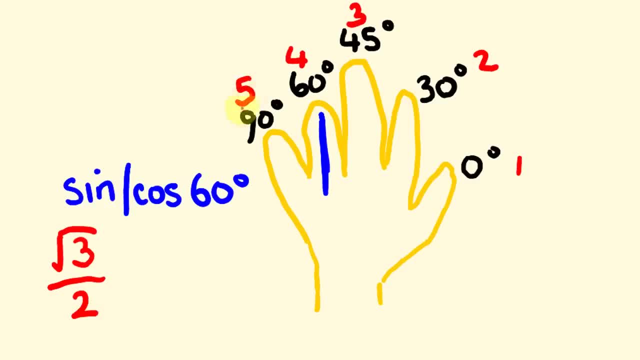 Okay, The cosine that's on the left-hand side. here there's 1 finger there. Okay, I'm going to square root it. so the square root of 1 is 1. And I'll put it over 2.. And that's all there is to it, right? 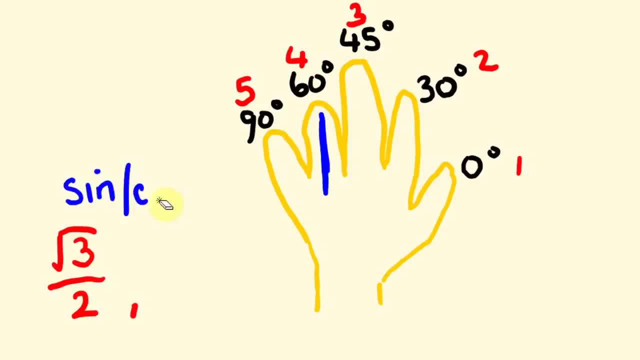 Okay, not bad right. That's a fairly simple trick. What about we go through another one of these? So what about we do? I want to know what the sine and cosine of 60. Let's say, let's do 0 degrees, Okay. So you're going to see here that we have, okay, I'll put my 0 degrees in here, Okay, And all the ones on this side are going to be our cosine and the ones on this side are going to be our sine. So pretty easy, right. 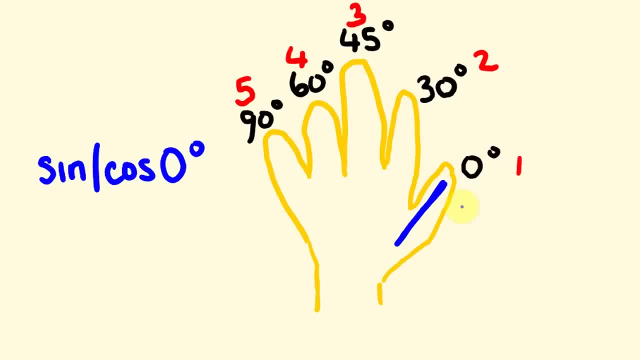 So sine first, You're going to see here that there's no fingers. Okay, so nothing. Alright, That's over 2, square root of nothing. So it's, we've got a nothing answer there. What we have here is we have 4 fingers for our cosine, The square root of those, which is equal to 2.. And we're putting that over 2.. So it's equal to 1.. 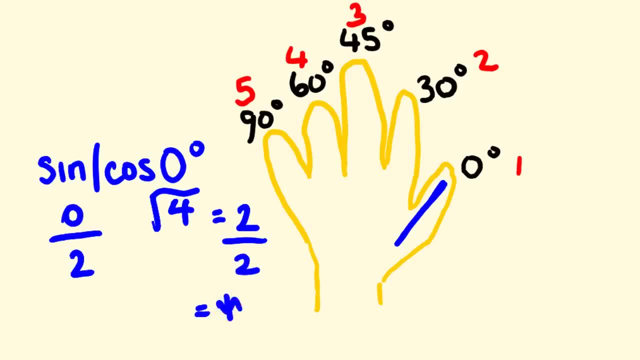 Okay, Told you this was going to be a nice simple trick. and it is a fairly simple trick. yeah, Carry this calculator around with you all the time. Okay, What about one last? one of these Say: we want to work out the. 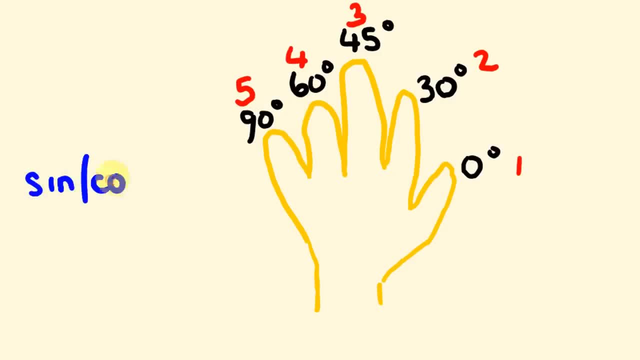 Sine and cos of the sine and cosine of 45 degrees: Okay, We're on the old middle digit there, Okay, So what we have is as follows: The sine- we've got 2 fingers here, Okay- 1, 2.. Square root of 2, over 2.. 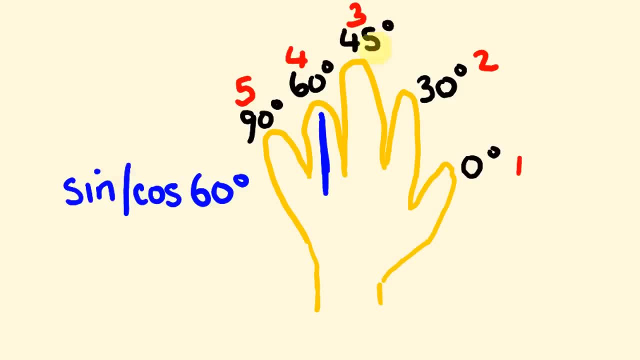 To say cosine of 60, sorry, the sine of 60, it's this: 1,, 2, 3 fingers here. Okay, on that side there's 3 fingers. So I get 3 fingers. I'm going to square root them and I put them over 2.. And that's our answer. 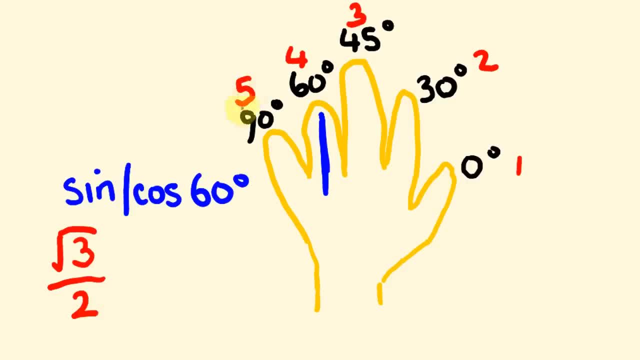 Okay, the cosine that's on the left hand side. here there's 1 finger there. Okay, I'm going to square root it. so the square root of 1 is 1 and I put it over 2.. And that's all there is to it, right? 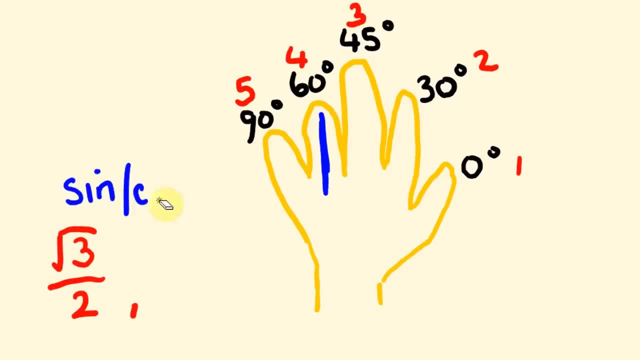 Okay, not bad, right, That's a fairly simple trick. What about we go through another one of these? So what about we do? I want to know what the sine and cosine of 60. Let's say, let's do 0 degrees, Okay. so you're going to see here that we have, okay, I'll put my 0 degrees in here, Okay, and all the ones on this side are going to be our cosine and the ones on this side are going to be our sine. So pretty easy, right. So sine first, You're going to see here, there's no fingers, Okay, so nothing, All right, that's over 2.. 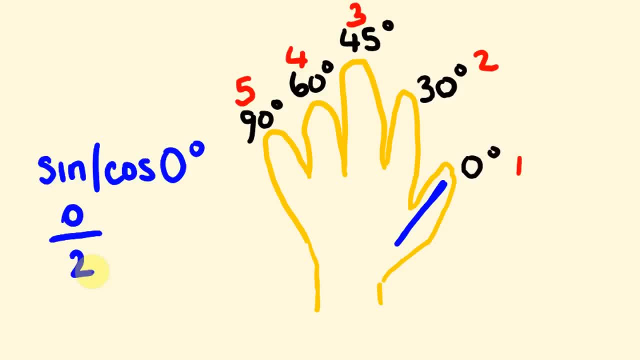 Square root of nothing. So we've got a nothing answer there. What we have here is we have 4 fingers for our cosine, The square root of those, which is equal to 2.. And we're putting that over 2.. So it's equal to 1.. Okay, 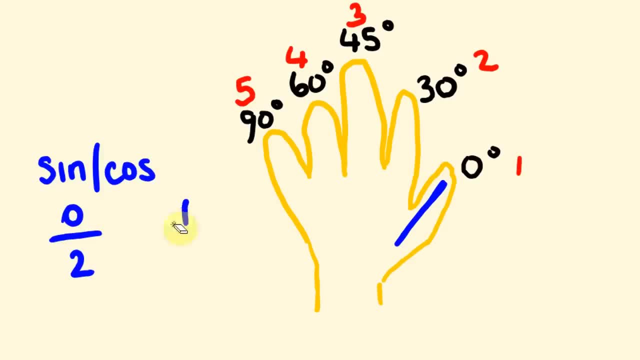 Told you this was going to be a nice simple trick. and it is a fairly simple trick. yeah, Carry this calculator around with you all the time. Okay, what about one last one of these? Let's say we want to work out the. 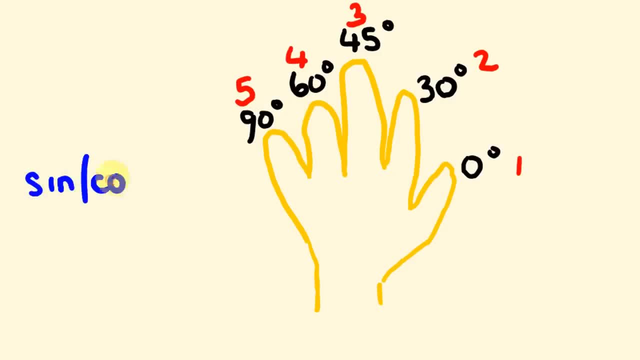 Sine and cos of the sine and cosine of 45 degrees: Okay, We're on the old middle digit there, Okay, so what we have is as follows: The sine- we've got 2 fingers here, Okay, 1, 2.. Square root of 2 over 2..